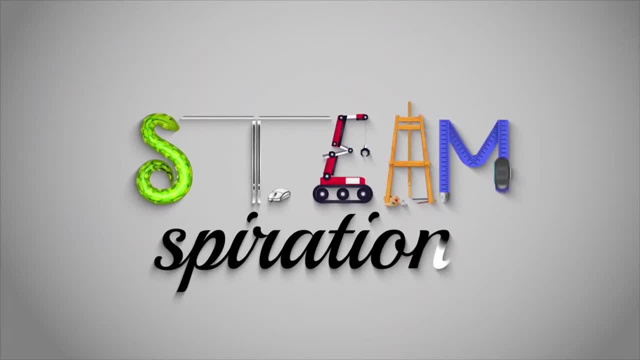 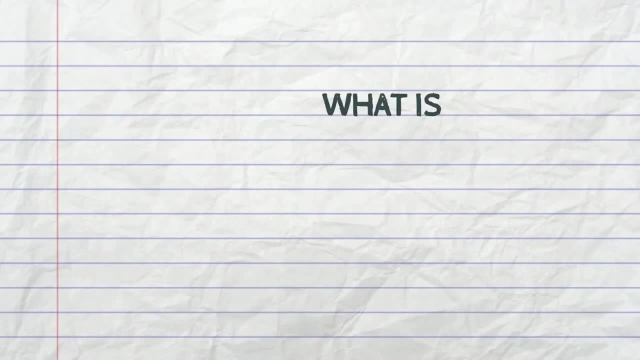 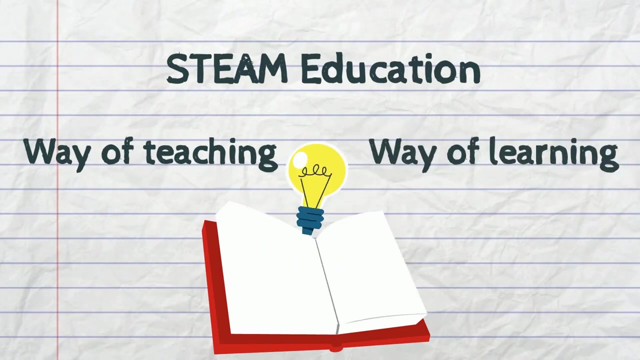 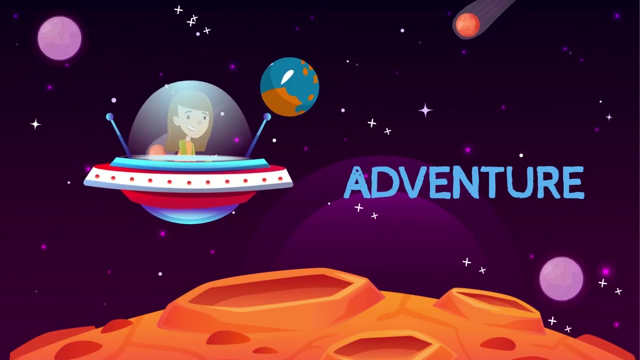 What is STEAM education? In a simple way to explain, STEAM education is a way of teaching and a way of learning that combines science, technology, engineering, arts and math. We can think of STEAM education as an adventure, where the most important part of our adventure is our. 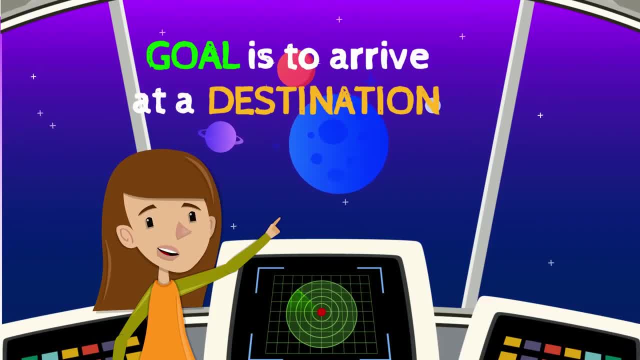 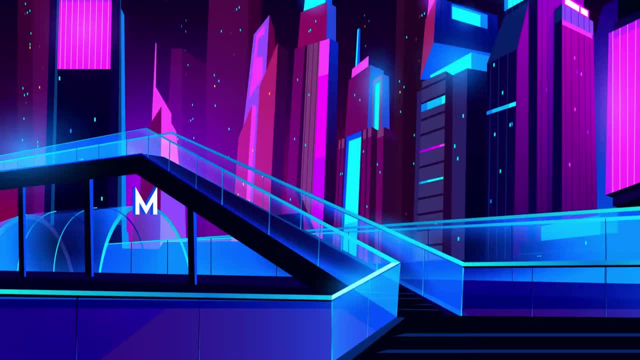 journey. Our goal is to arrive at a destination, but how we get there and the roads that we take are different for everyone, because we all think very differently. Along this road, we make mistakes and sometimes we get lost, but this is where we learn the most and this is where we begin to. 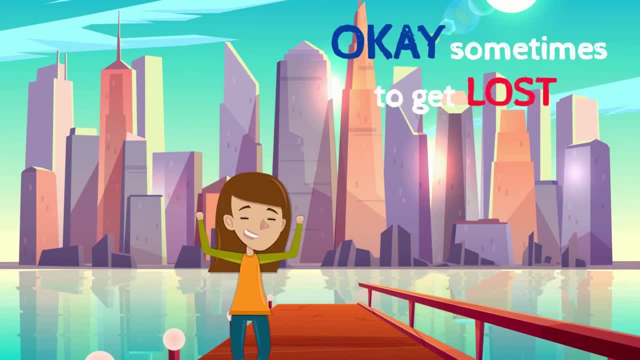 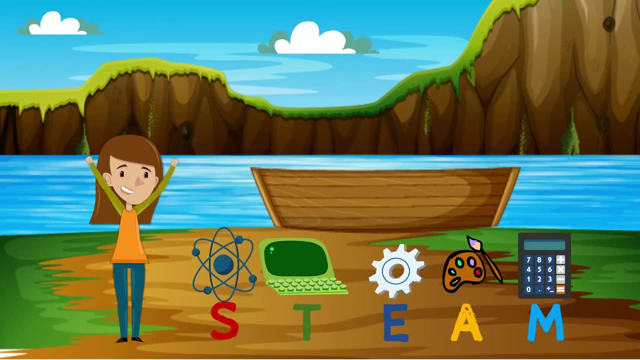 understand that it is okay sometimes to get lost. Our friends on this road are science, technology, engineering, arts and math. They guide us to our final destination. Some friends are closer to us than others, so we might like to ask our math friend for help, or maybe our engineering friend. 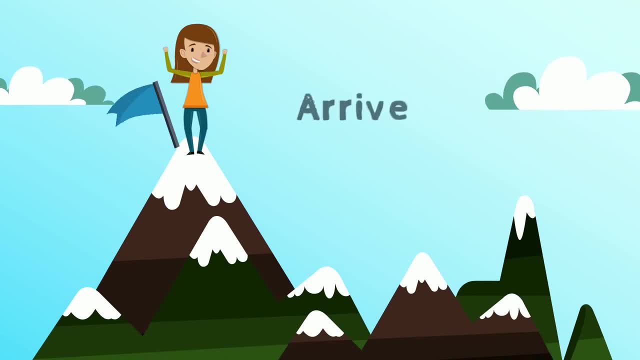 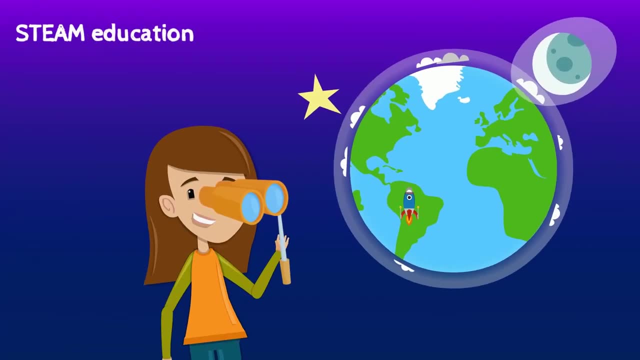 but in the end we become best friends with everyone. When we finally arrive at our destination, we discover that it is not the end but the beginning to more questions and more adventures. STEAM education inspires us to explore the world and see it differently. It helps us to learn in. 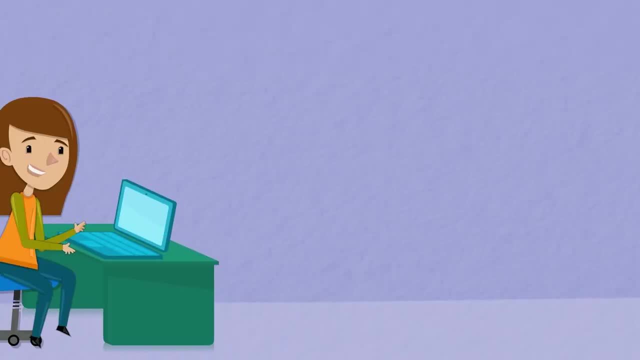 a fun way and work with each other to solve problems and take risks, learn from our mistakes and change the world. As STEAMspirations, we are about teaching, learning and learning. We are about teaching, learning and learning. Teachers, parents and students: we are all about you. 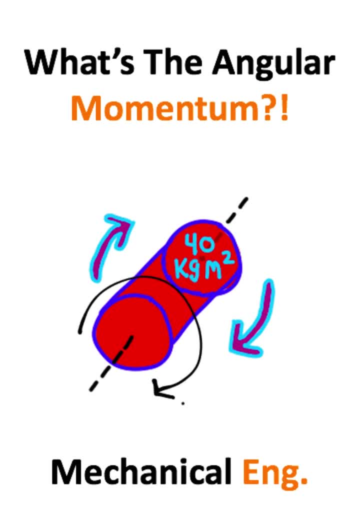 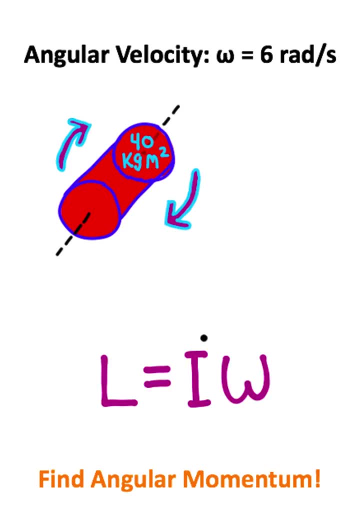 We have a large cylindrical can spinning on its axis of symmetry. We want to calculate the can's angular momentum. So to calculate the magnitude of angular momentum, what we want to do is take the product of rotational inertia and angular velocity. The rotational inertia is provided for us in this problem. as 40 kilogram meters squared, The magnitude 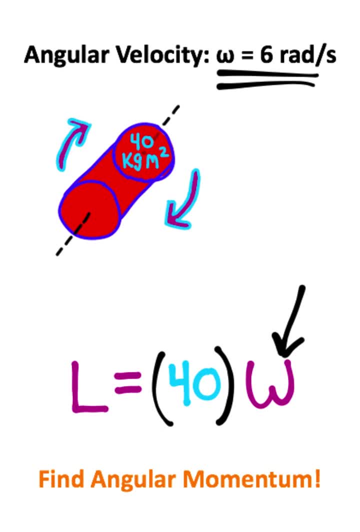 of the angular velocity is also given to us as 6 radians per second. So the magnitude of the angular momentum is going to be 40 times 6, which comes out to 240.. And multiplying these units by these units, we get 240 kilogram meters squared radians per second, And that